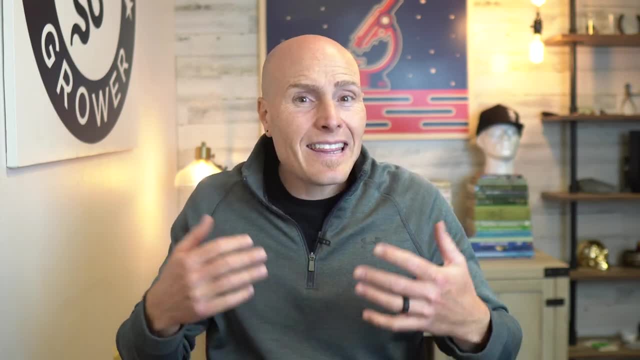 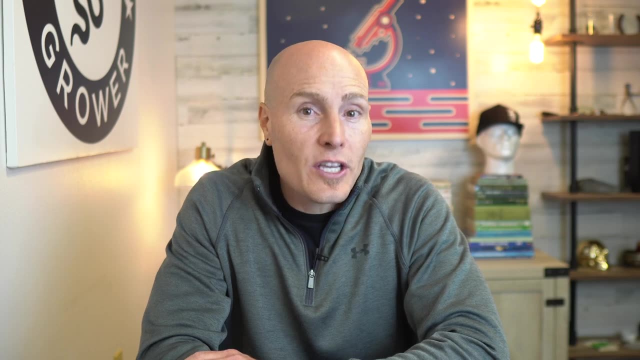 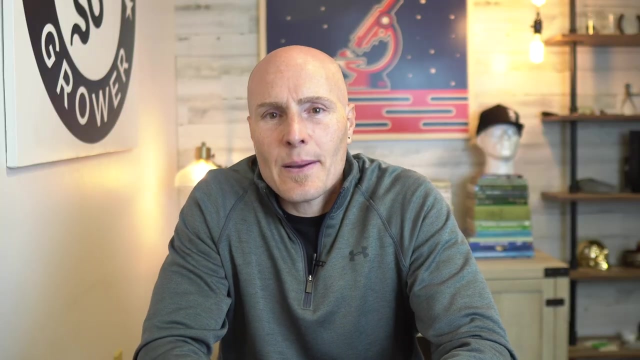 Soil texture and soil structure. You might think they mean the same thing, but they're actually very different. Let's look at how they're different and why it's important to you as a gardener. Thanks for watching the video today. I'm Diego D-I-E-G-O, and my goal is to help you streamline. 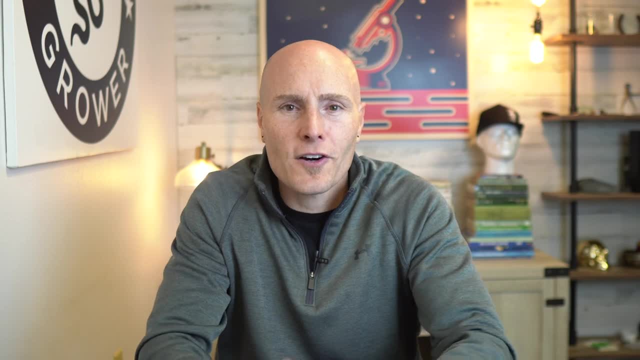 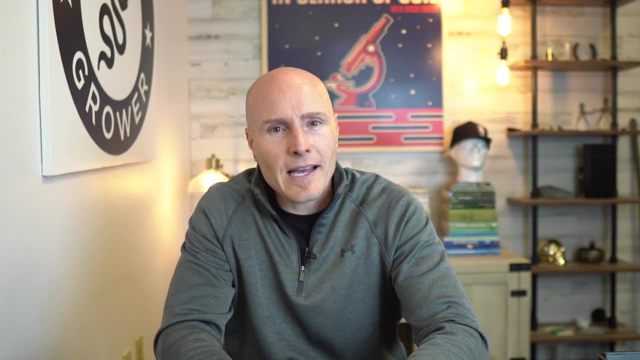 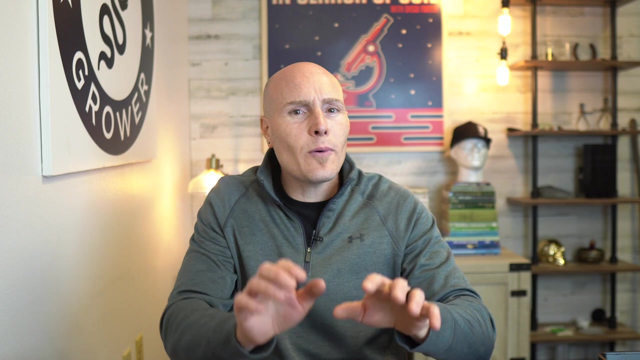 gardening to work smarter, not harder, using smart design. Soil texture versus soil structure. I'll be honest, when I started looking into this topic, I didn't really know the difference between them, And I'll ask you before I get into this video: do you know the difference? 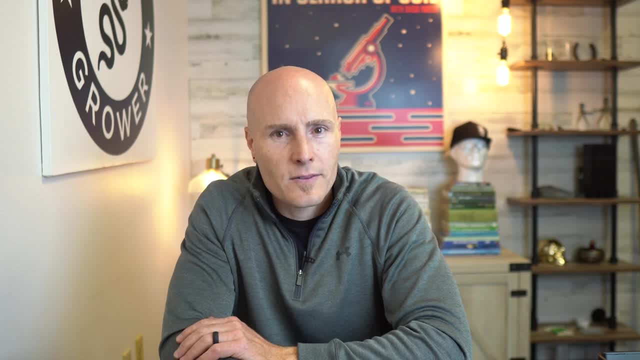 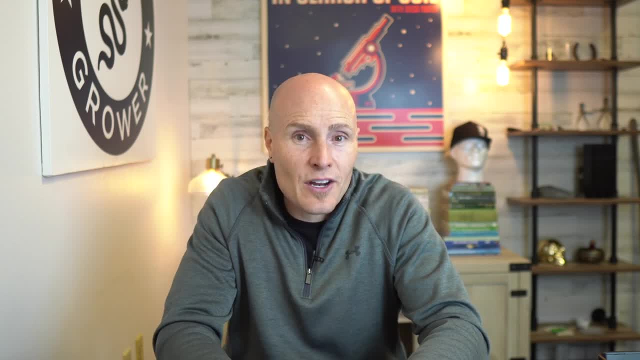 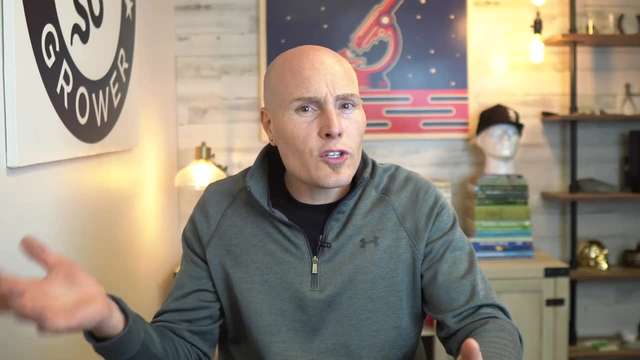 is the physical mechanism of soil structure. Soil texture is the physical mechanism of soil structure. soil structure is how that mixture comes together in the ground: loose, blocky, granular or solid. both soil texture and soil structure combined to determine how plants grow in the soil. 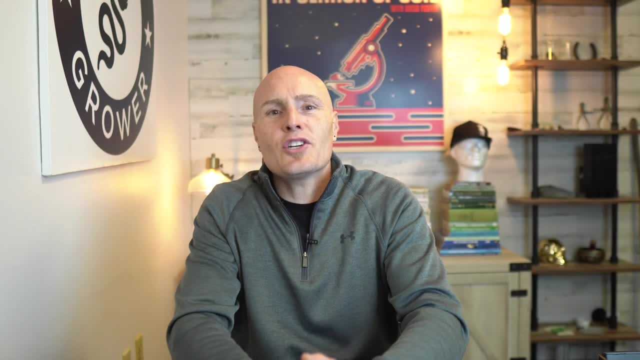 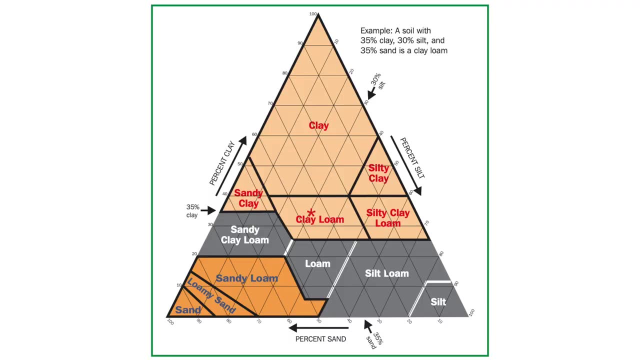 so let's take a closer look at each soil. texture is based on the mineral makeup of soil, as shown in the soil triangle. the soil triangle is a matrix to help you classify your soil. on each corner you have sand, silt and clay. you would analyze your soil and determine the percentage of clay, sand and 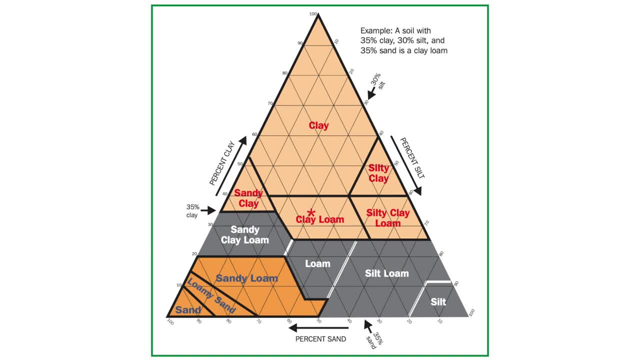 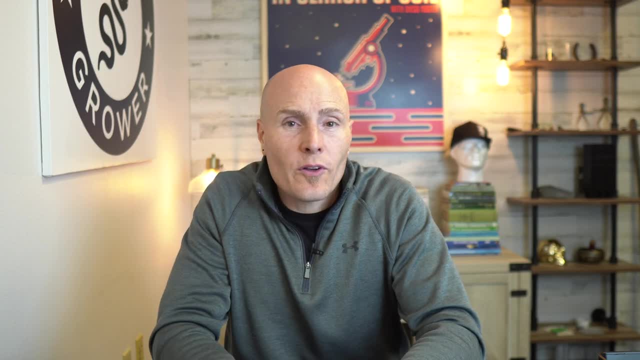 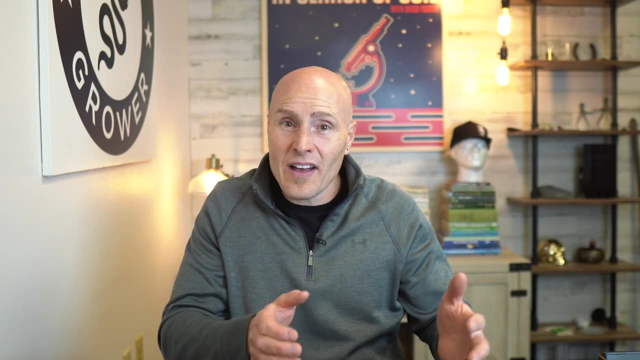 silt and that would put you somewhere in this triangle and, based on where you land in the triangle, that's how you would classify your soil. the ideal agricultural soil is what's known as loam. that's the perfect mixture of sand, silt and clay. it's about 75 percent combined sand and silt. 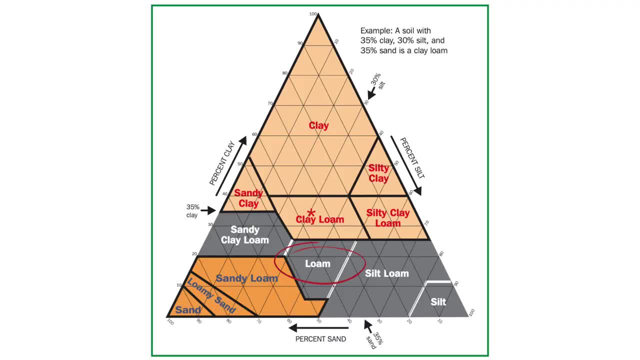 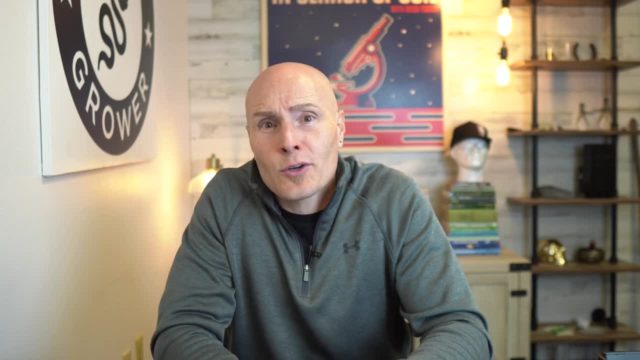 and 25 percent clay and you can see that loam sits right here in the soil triangle. why is loam so good? why do we want loam in our garden and why do gardeners who have loam in their garden brag about it? it has to do with the particle size. 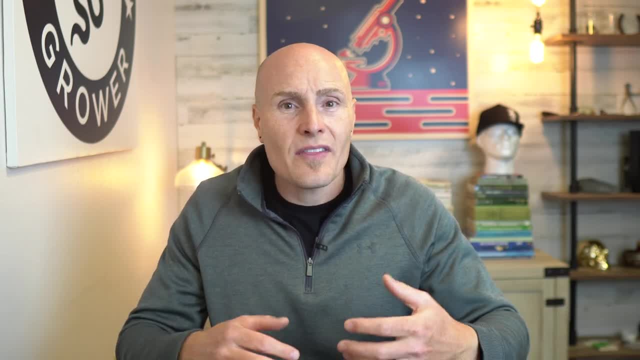 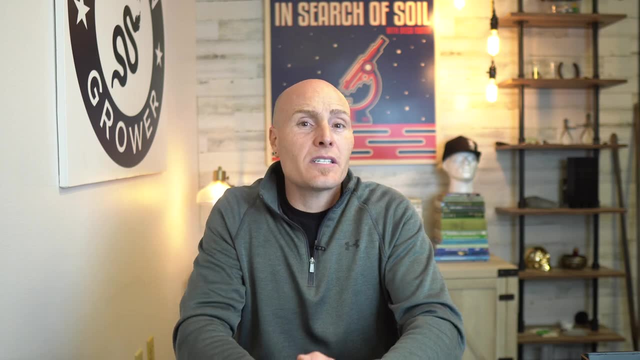 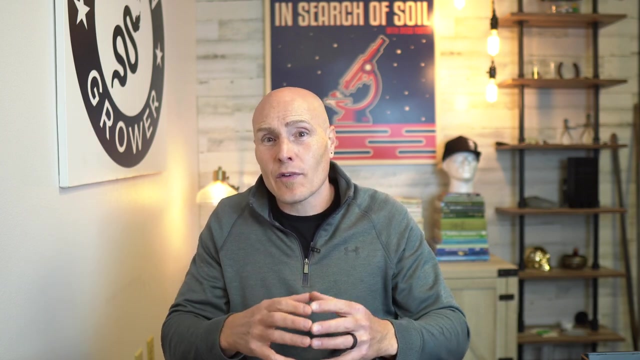 and the properties of each of those minerals that makes up loam, sand, silt and clay. sand, silt and clay are all different sizes. sand is about a thousand times larger than clay and about 40 times larger than silt. this size differential is what accounts for poor space. 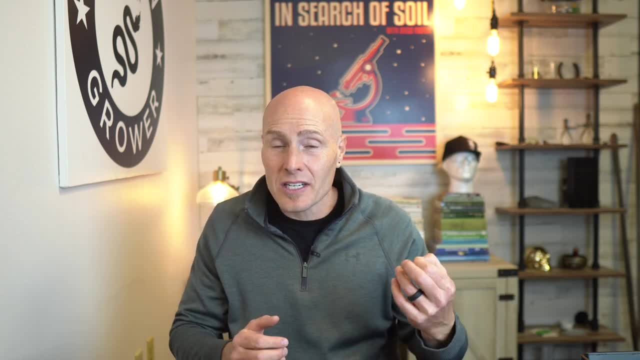 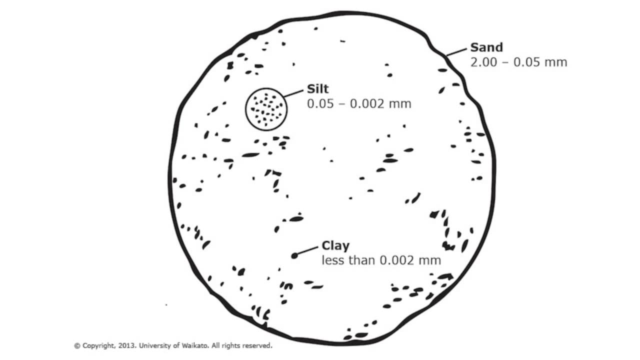 in our soil. poor space is needed because that's where oxygen, biology and water can flow through the soil and be stored in the soil. you can see a representation of the size of sand, silt and clay in this diagram here. the smaller the particle size, the tighter the soil and the harder it is for air. 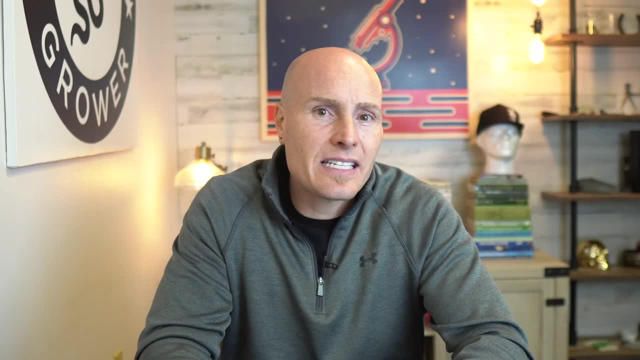 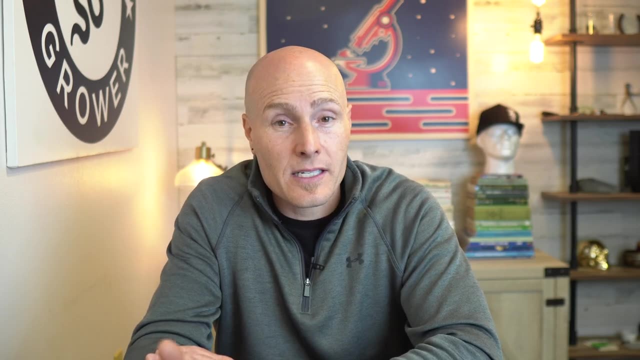 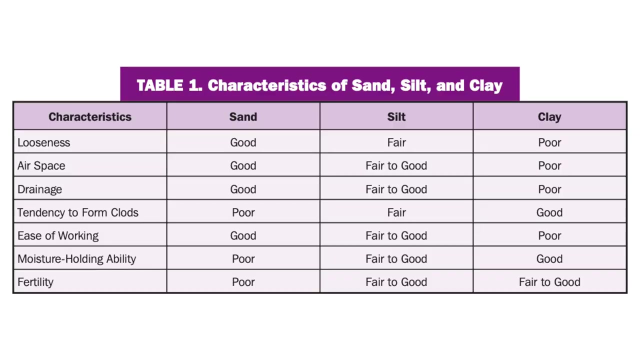 water and roots to penetrate the soil. the size of sand, silt and clay isn't the only property of those three components that affects how well soil can grow plants. there's other characteristics of each of those three components that help determine the value of an agricultural soil. if we look at this chart here, we can see some of the pluses and minuses. 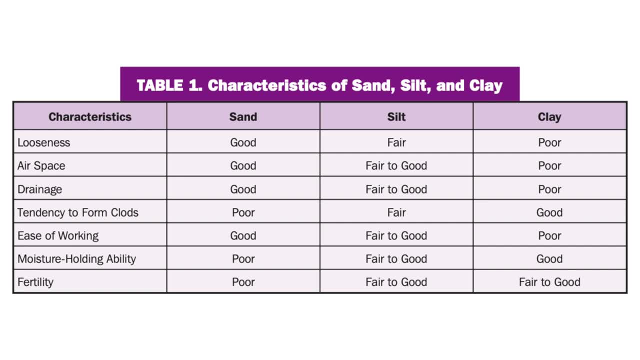 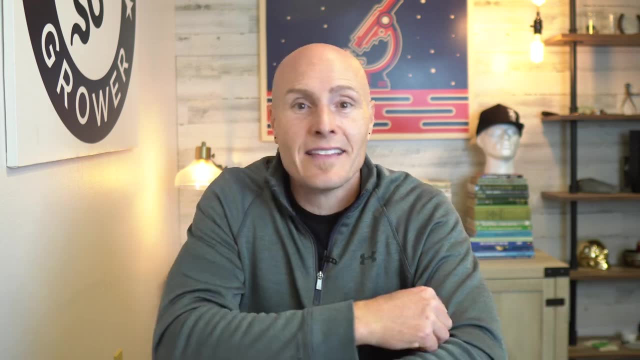 of sand, silt and clay. for example, if you want a soil that drains well, you want a lot of sand. you don't want a lot of clay. if you want a soil that holds water really well, you want more clay relative to sand. the optimum mix for agriculture is some sand, some clay and some silt, and that's. 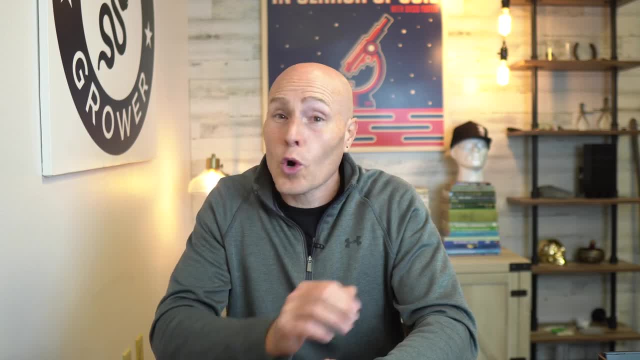 known as loam, and that's the difference between sand, silt and clay. the optimum mix for agriculture is some sand, some clay and some silt, and that's known as loam- loam- Without knowing your soil texture or without knowing the mineral makeup of your soil. 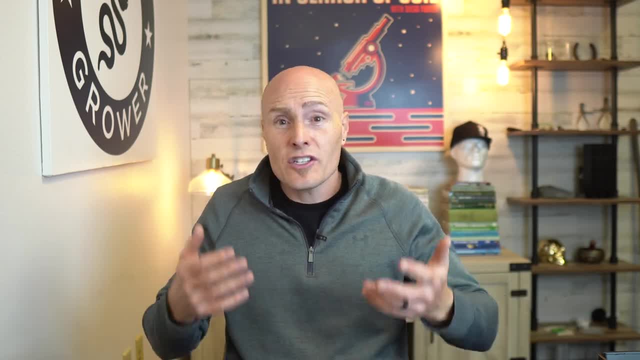 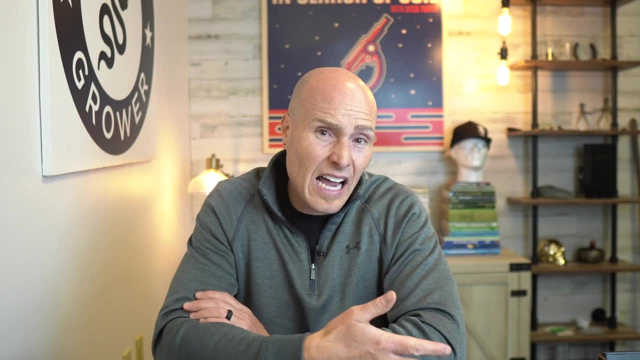 you can probably have some sense of what your soil texture is. Just think about your time in your garden. How easy is it to dig through it when it's reasonably moist, meaning not too dry, not too wet? If it's really hard to dig through your soil, then you probably have a tighter soil. 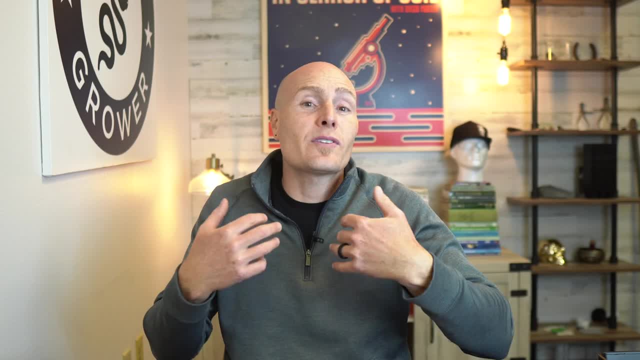 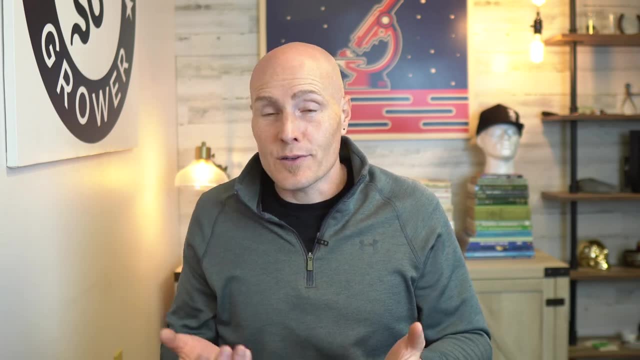 that lends more to the clay side of things. If your soil is very easy to dig through, then you probably have a sandier soil. So when you dig, do you get clods or do you get loose sand? If you get clods, you have a lot of clay, And those clods are known as soil aggregates. 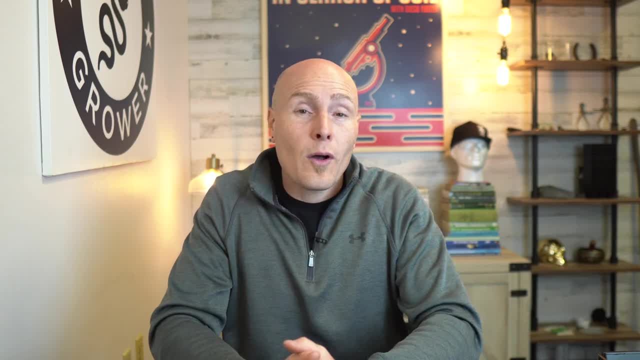 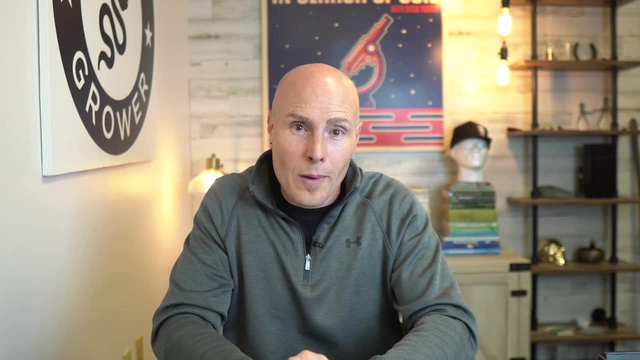 Aggregates are when a bunch of smaller particles come together to form a larger particle. Think a snowball that you might be making right now. You take a bunch of small snowflakes and you aggregate it into a snowball that you throw at your friend or at a school bus and end up getting 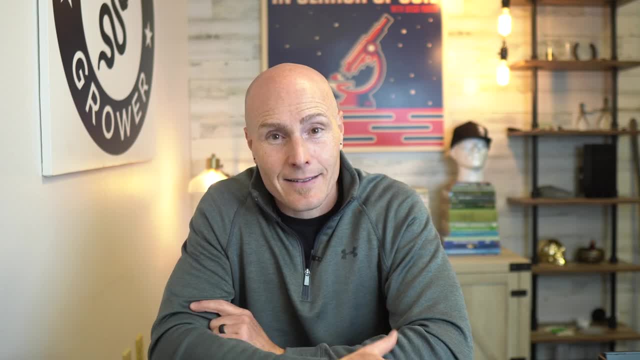 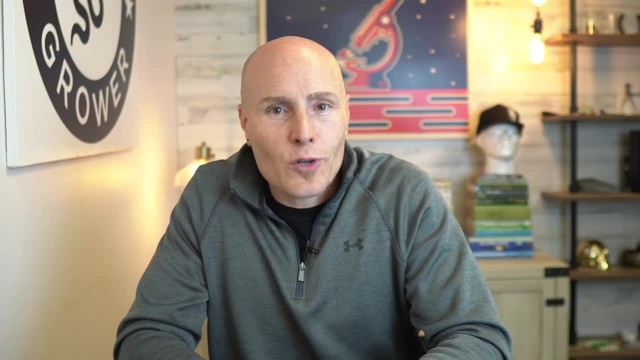 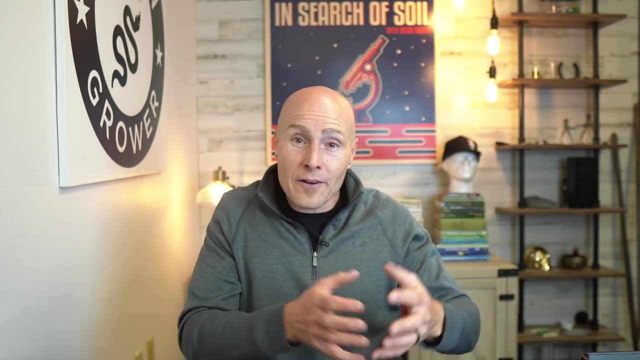 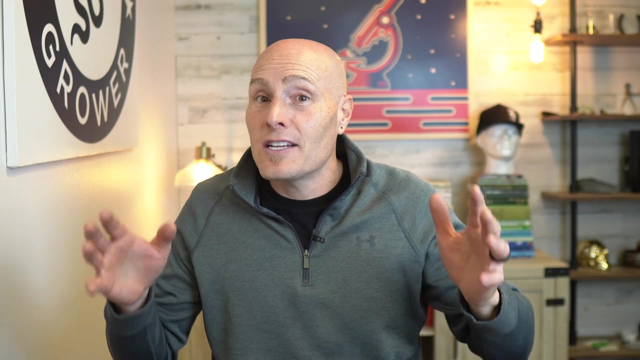 soil. Soil aggregates themselves are what make up soil structure. So here's where we go, from soil texture to soil structure, How sand, silt and clay come together to form aggregates. that is your soil structure. The proportion of sand, silt and clay doesn't matter at this point, It's just. 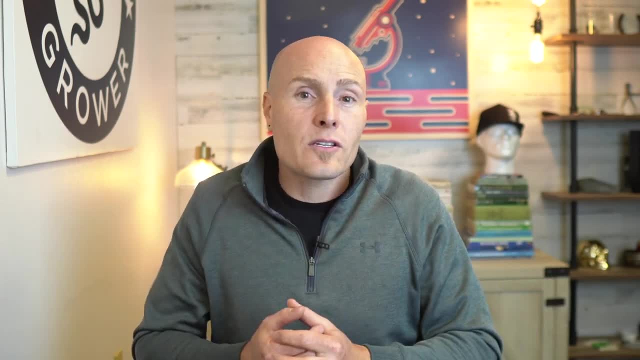 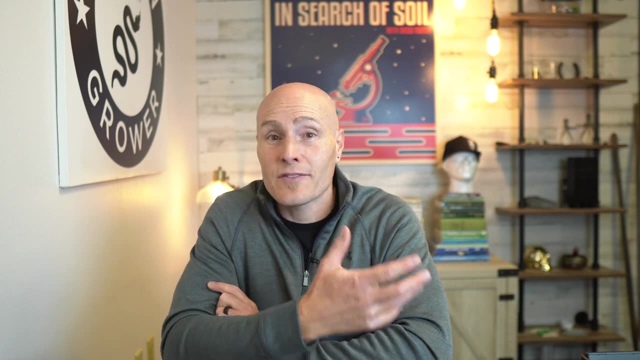 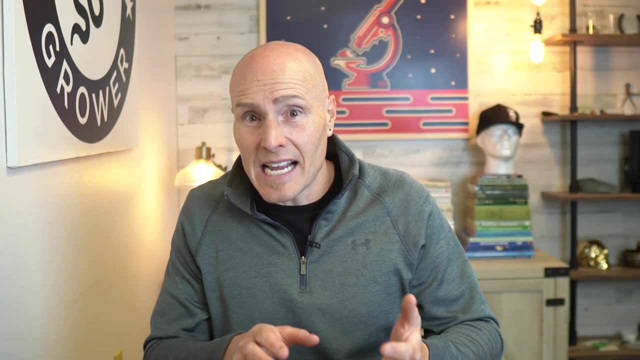 how all those three components come together. What do they form in the soil? Loose, granular soil or blocky soil, And that is known as soil structure. That's the arrangement of soil particles into aggregates of different sizes and shapes. We'll look at the different aggregate shapes and sizes. 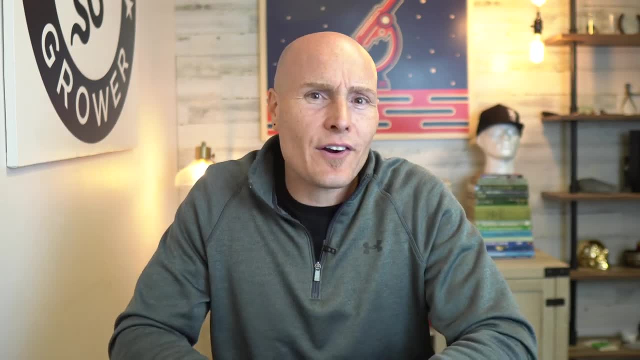 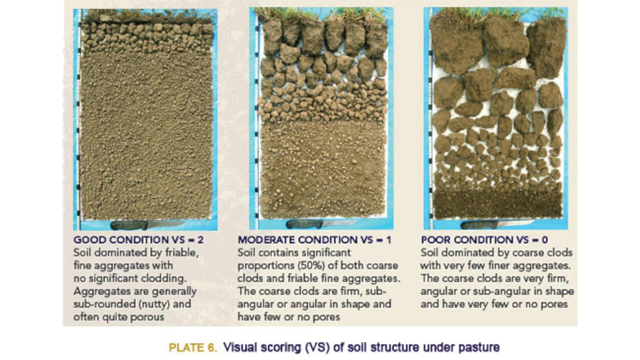 in a moment. but why is that important? Why should you care as a gardener? Soil structure affects water and air movement in soil, nutrient availability for plants, root growth and microorganism activity. The pore spaces created by those aggregates in the soil known as clods. 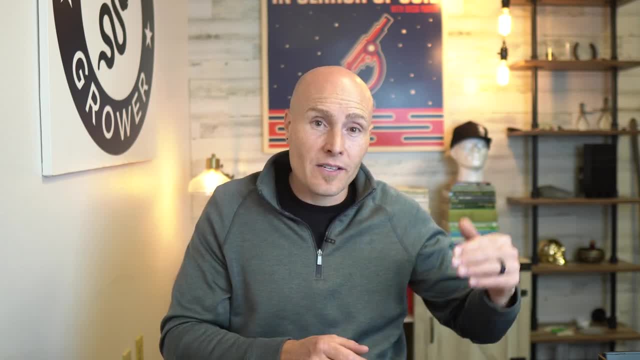 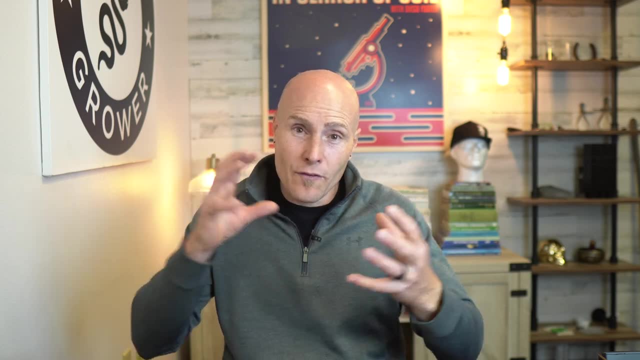 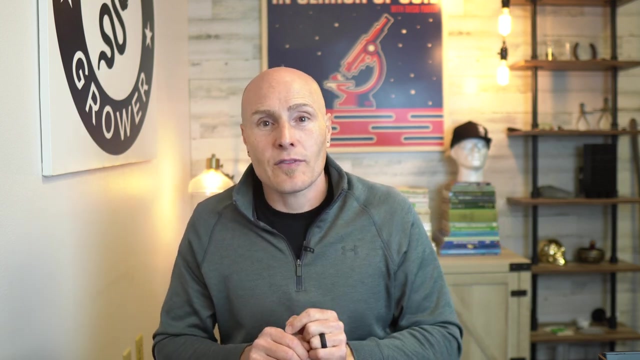 they're larger than the pore spaces of individual grains of sand, silt and clay. Bigger particles, bigger pore spaces. So if you take a bunch of sand, silt and clay and you form it into a ball, the pore space between each one of those balls is going to be much larger. That is a larger space. for roots, biology, water and air to go through. That's why you want larger pore spaces in your soil. to a certain extent, Too much is bad, but you want enough- versus a heavy clay soil which doesn't have much pore space at all and doesn't allow your roots to penetrate through it. Here's: 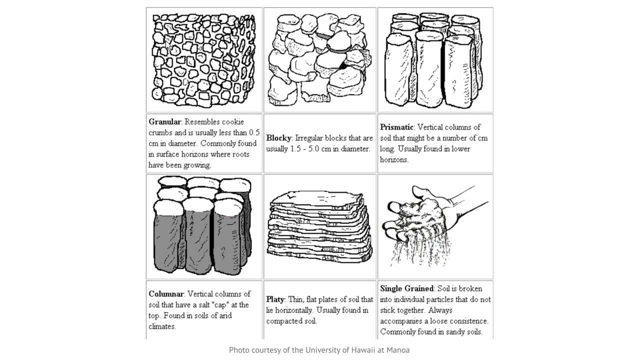 some examples of soil structure. The key here is: you're looking for a granular soil structure that's going to be loose, like cookie crumbs or coffee grounds. Just think potting soil. Look at how loose potting soil is. They make potting soil like that for a reason: because the roots can penetrate it. What would 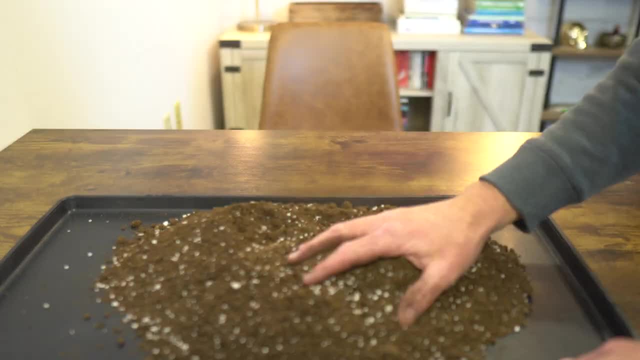 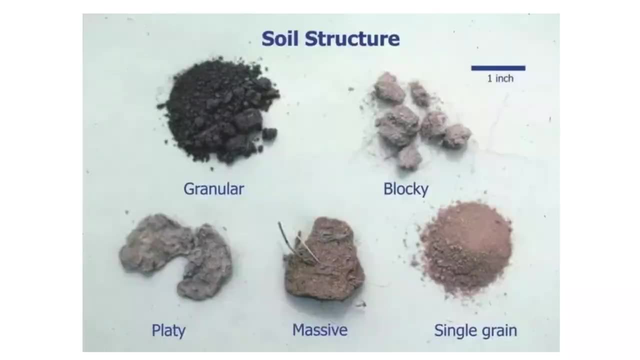 you rather put your hand through Potting soil or a stack of dinner plates? You'd choose the potting soil. Here are some different pictures of those soil structures in reality: Granular, blocky, platey, massive and single grain. 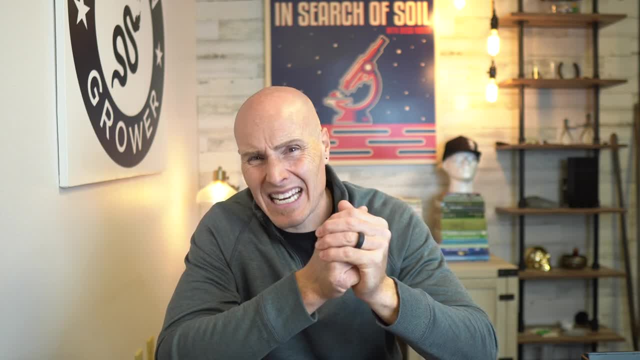 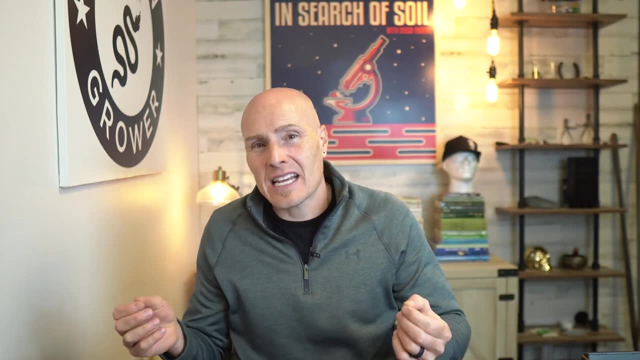 You might be thinking that single grain is the way to go. but that's like sand at the beach: It's too loose, There's no structure to it whatsoever. You're looking for a granular soil that brings together some of those smaller grains into larger aggregates, but not too large, so you don't get. 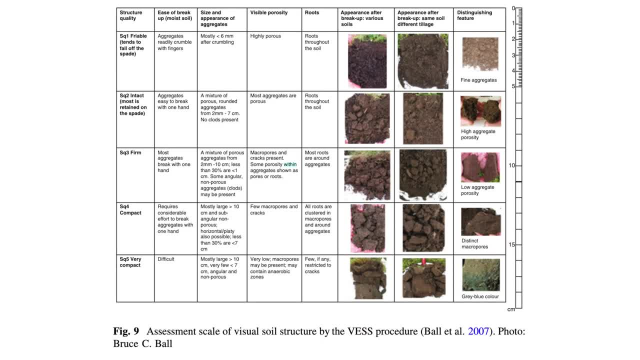 large blocks. I'll leave this slide up here for a minute. This is some extreme nerdery. If you're into your soil and analyzing soil structures, take a look at this slide and see how soil structure affects root growth, As you can see here, friable. 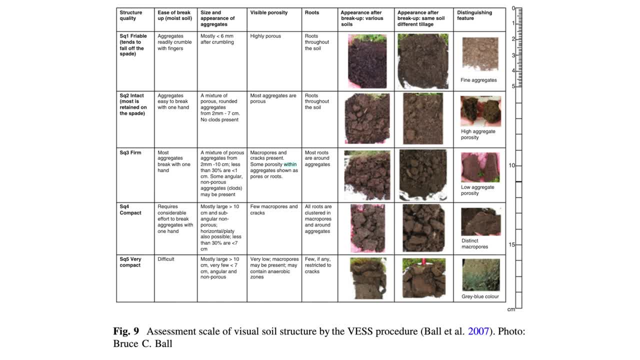 loose sites are growing a lot. These are broken down in the sensible direction so that you can spot large bills of soil Again. this is not a bridge that's pursue by, of course, all 하지만 that part that's very much contact but light. This is a very rich foundation for soil structure. 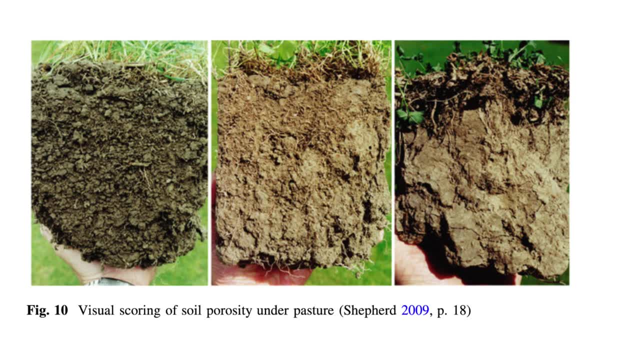 Here is one more example in Figure 10, showing a pasture with three different types of soil, With the best soil being on the left, a more granular soil, vs the soil on the right, more blocky or massive chunks, and you can see the darker soil is the one on the left. 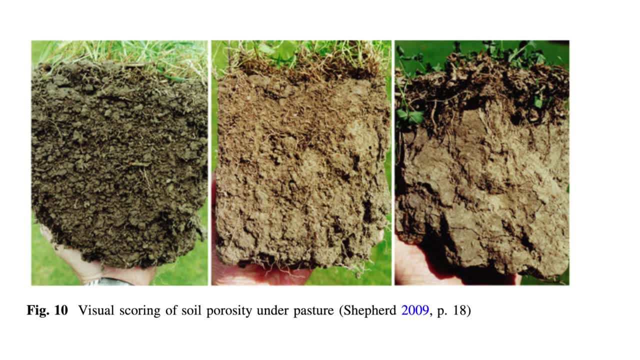 alluding to more biology, more root growth vs the blockier, more massive pooply soil right block on the right, which probably has plants struggling to grow on it. what you don't want in your garden is the one on the right and what you want is the one on the left. so how do you make? 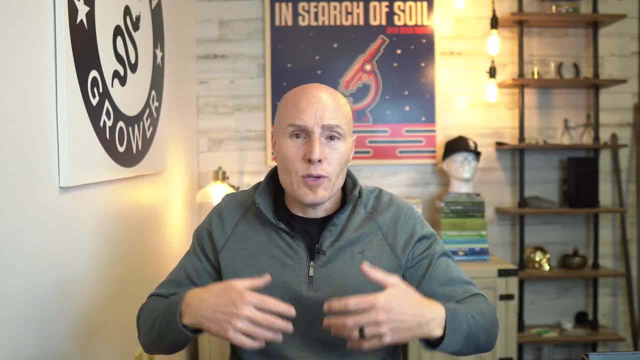 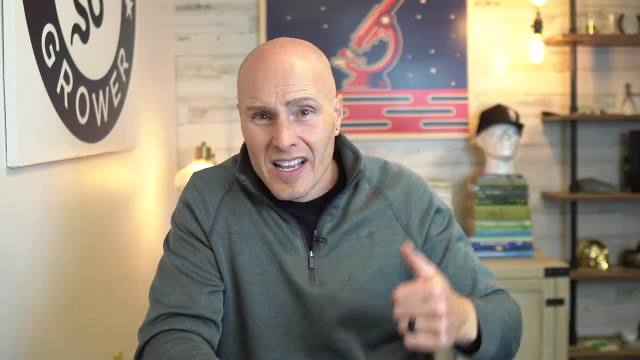 good soil structure initially. you can do it by fluffing it up. you can add moisture to the soil, you can add plants to the soil and on the flip side, there's a lot of ways to ruin soil structure: tillage, compaction, letting the soil dry out, removing organic matter, removing plants from. the soil. all of those things force the soil to tighten up. when it tightens up, you get larger and larger aggregates that form. the larger the aggregates that form, the harder it is for the roots to penetrate through those aggregates themselves. so keep plants in the soil, don't. 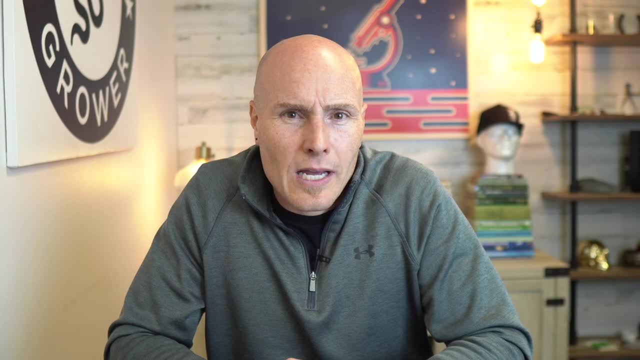 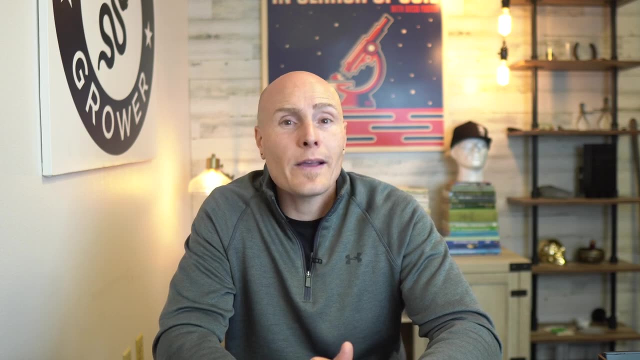 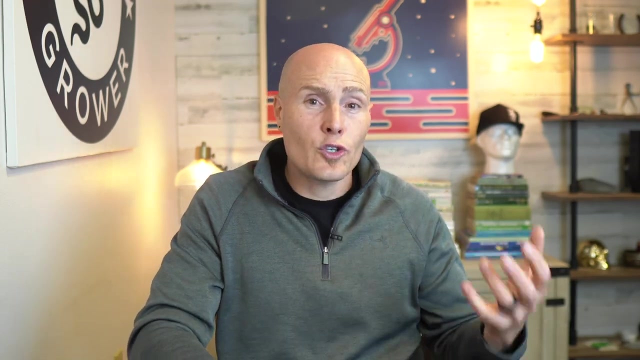 till and you'll probably have pretty good soil structure in no time. this is why you avoid walking on your beds excessively, driving over them. it's why you avoid tillage and why you should always keep plants in the soil for as long as possible. all of this affects how plants grow, not just from.